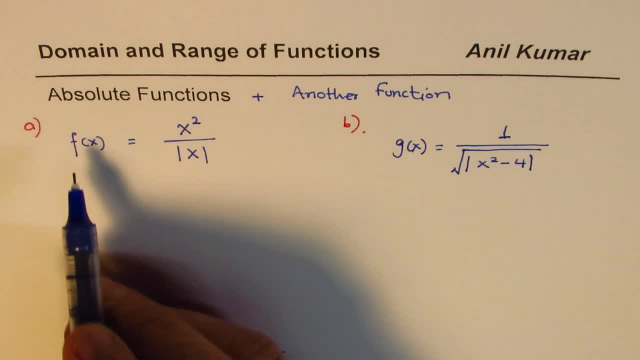 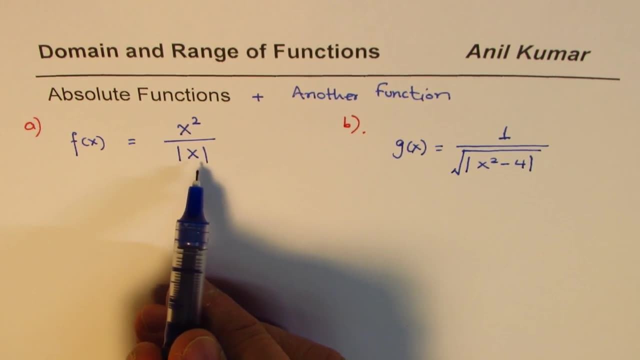 into my suggestions. Let's begin with the very first one, which is f of x equals to x square divided by absolute x. Absolute x is actually a piecewise function which is also defined as: absolute x equals to positive value of x if x is greater than equal to 0, and just negative value of x if x is less than 0.. 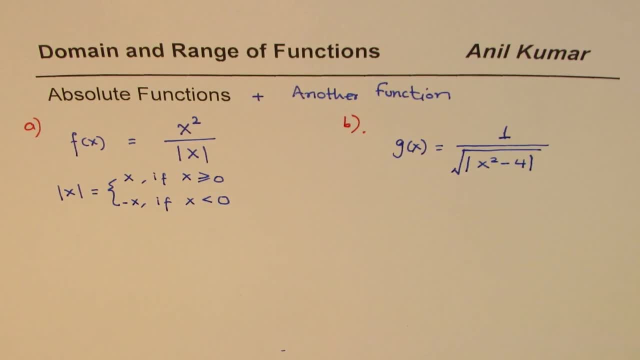 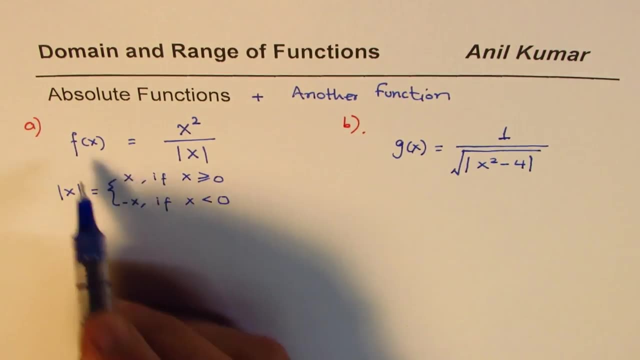 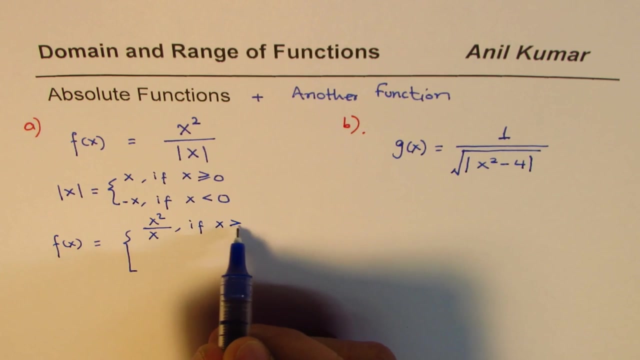 So this definition will be used to redefine our function. So since the absolute x is a piecewise function, we could redefine the function f of x as equal to a piecewise function. See where it could be: x: square over positive x if x is greater than. 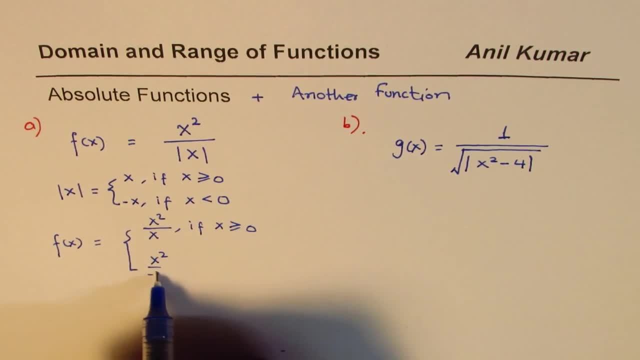 equal to 0 or it is equal to x. square over negative x if x is less than 0.. Now it is important to note that absolute x is in the denominator, So x is not equal to 0.. Perfect, Since x is not equal to 0 when we 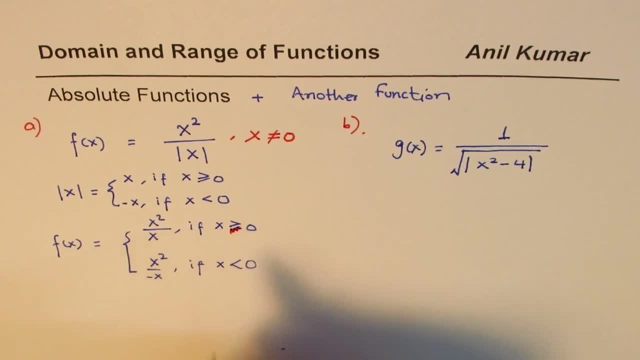 redefine our function f of x. we should not include this equal to right. So I purposely do it so that it is a constant reminder to you that when it is in denominator you should not include equal to sign here while defining the function right. I would have straight away written it, but you 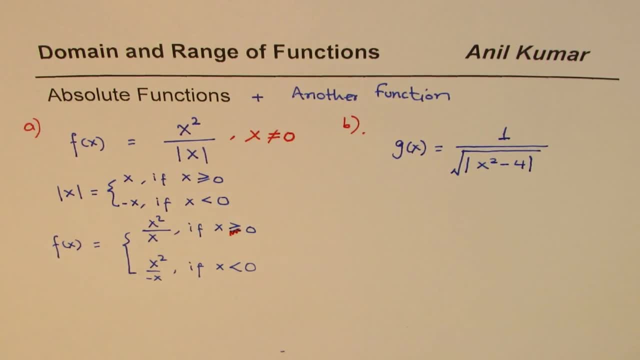 would have overlooked it, and that's the whole idea. So keep an eye on this. Whenever you do this, remember x equals to 0 is not in the domain of this particular function. Perfect, right. Okay, now to find domain and range of this function, let's go one more step and we'll write the function as equal to x. 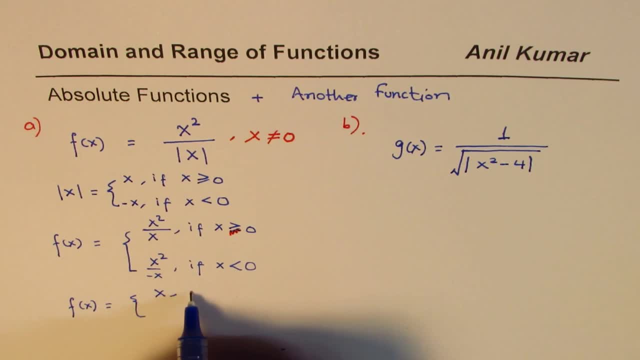 square divided by x is what It is: x, right? So it is x if x is greater than 0.. So I'm mistake. now that was on purpose. this one is minus x. if x is less than 0, you get it. so that becomes: 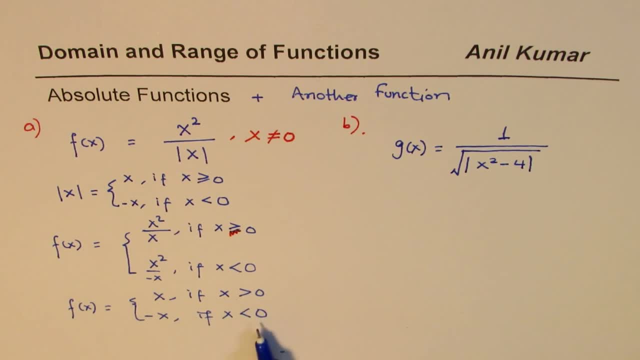 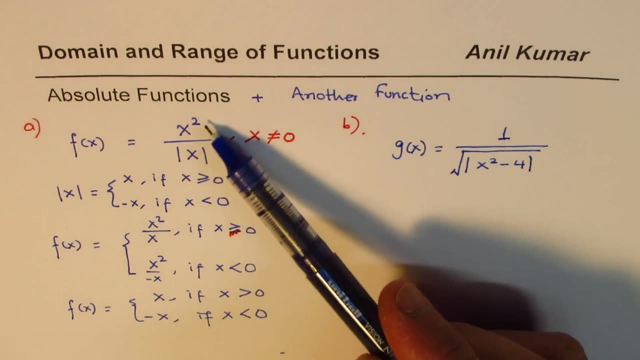 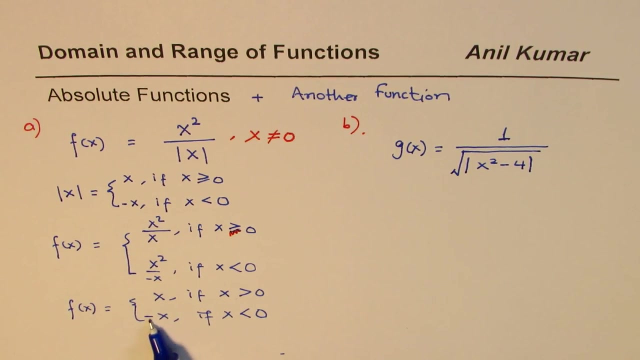 the the function. right? so if x is less than 0, it is minus x. well, if you see this equation, you will note that this function is always positive. do you see that it is always positive? so even though it seems to be negative, it is not really negative, right? that's the tricky part and that's the reason. 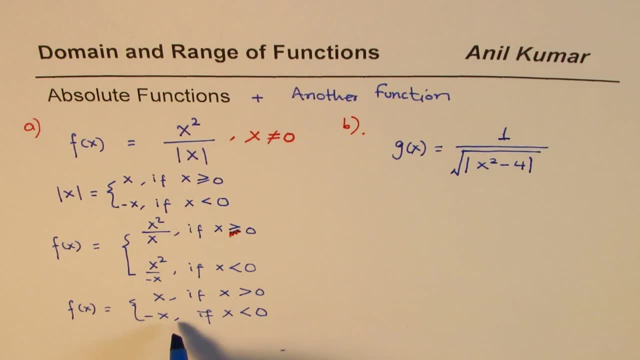 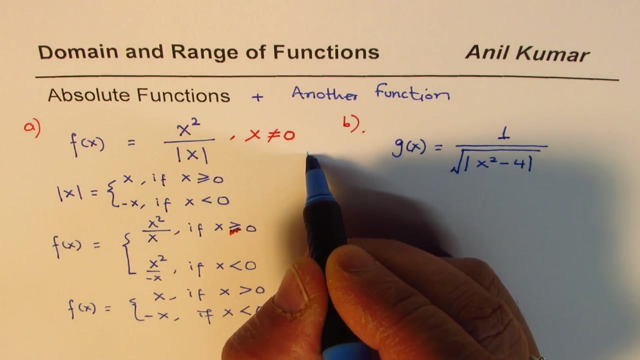 of my taking up this example. it really creates a lot of confusion. so let me sketch this before i get into domain and range. right, it seems as if range is all real numbers except zero, right? but okay, let's sketch it now. if you sketch it, what you really get here is: 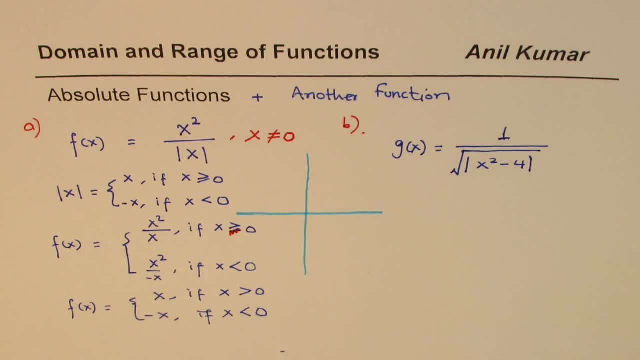 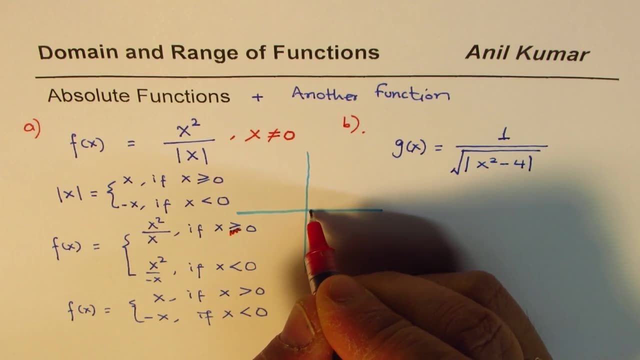 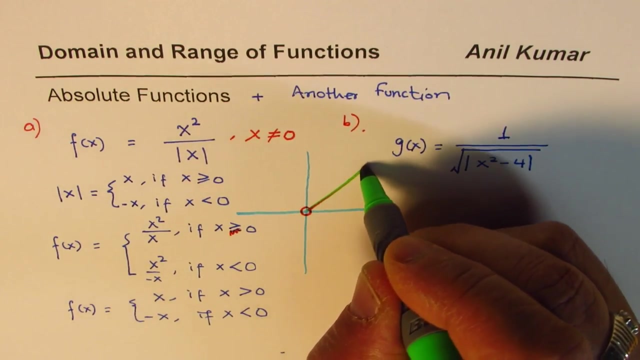 you that the right side is okay when x is greater than zero, then you know, it is like a straight line and this point is a hole right. so that is not in the domain of the function. this side is is kind of a straight line right. how about the left side? will it go like this or like that? 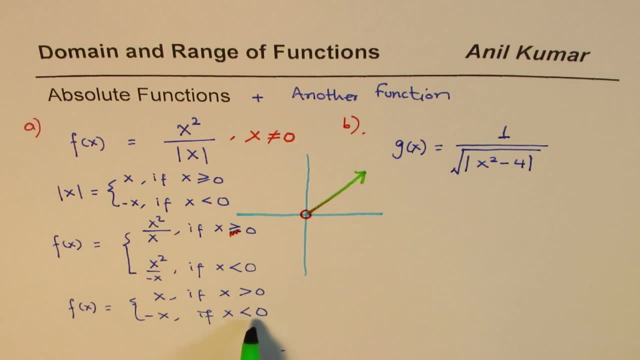 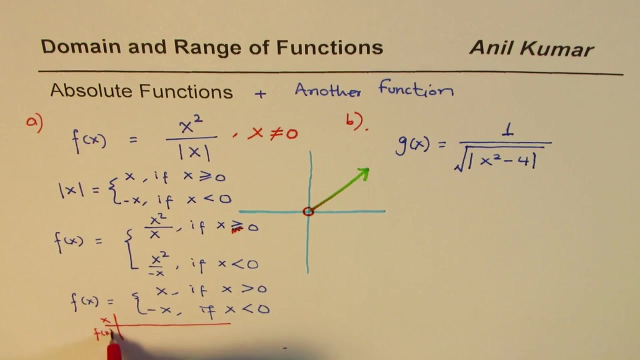 minus x if x is less than zero. so better is just place some values right. so let's place some values. so if i write x as, let's say, minus one, so let me write x values and f of x values. so if i write here minus one, so so minus of minus one will be plus one. do you see that? 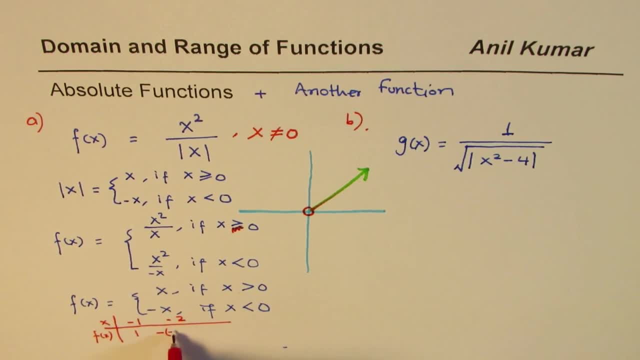 i'm going to say, if i write minus two, then minus of minus two is plus two. so at minus one it will be plus one, at minus it will be plus two. so basically on this side also it is going to be like this. so it is an absolute function which is actually not defined at zero, correct? so that 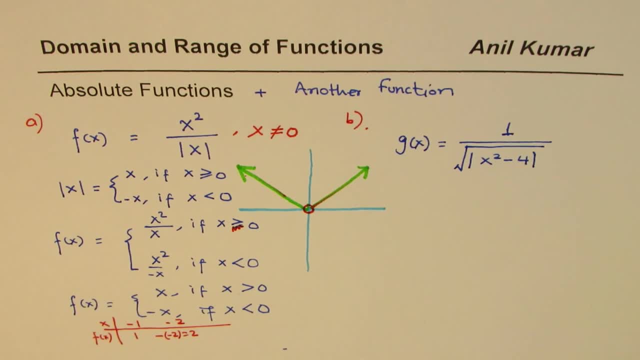 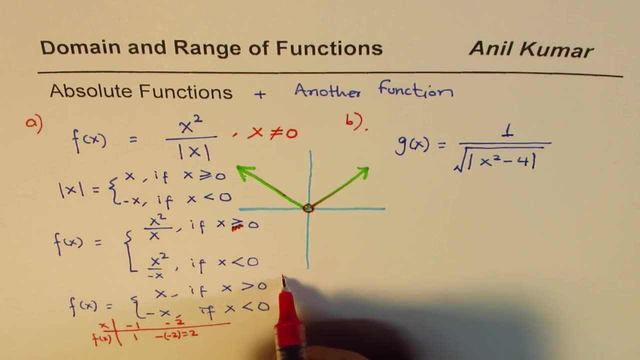 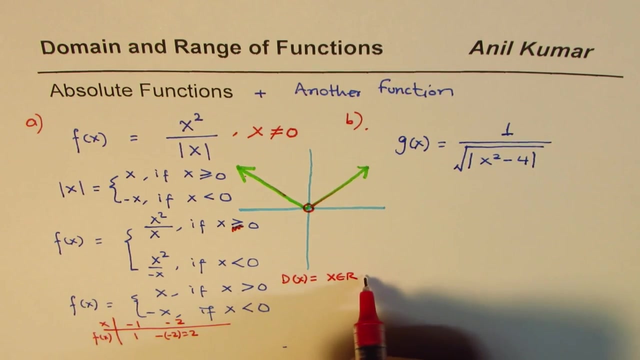 i hope helps you to write down domain and range of this function correct. so let me squeeze in the domain range for this function. now. we say domain of this function is x belongs to real numbers, where we can write this line: x is not equal to zero, is it okay? 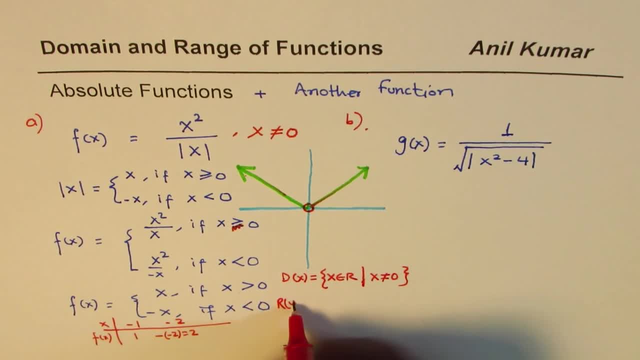 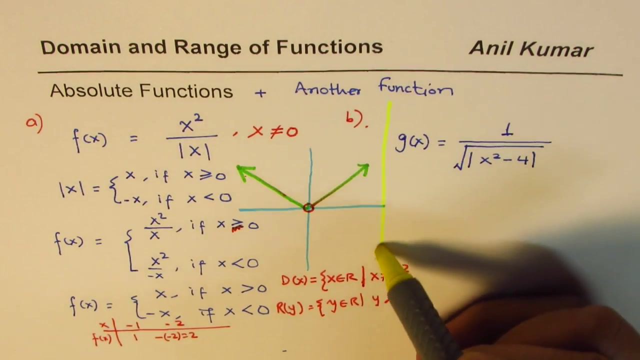 so that's the domain of this function and range for this function is: y belongs to real numbers. where y is greater than zero, it is also not equal to zero, so that becomes the domain and range of this particular function, right? so we took a lot of space from the next question into this one. 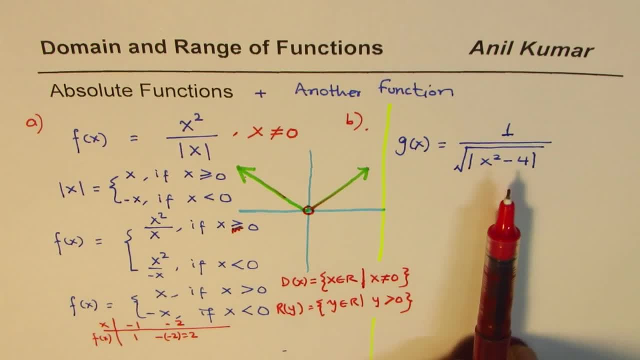 so i'll kind of squeeze in the solution for this one, okay, so now i hope this part is clear to you, right? so when we combine absolute function with other functions, things really change. x squared divided by absolute x is kind of absolute x where it is not defined at origin. 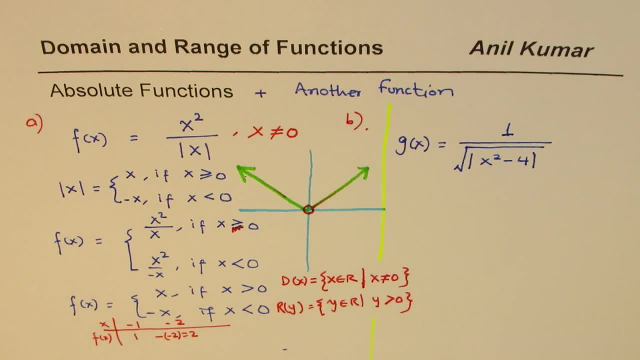 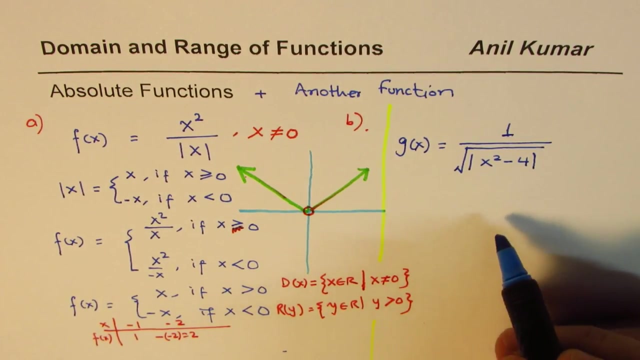 but otherwise it is same. okay, the next function is: g of x equals to one over square root of absolute value of x squared minus four. now here, instead of defining like this, i will use a different approach. we'll actually graph this and from the graph we'll draw, i mean, our conclusion about the domain and range. okay, so i'm just figuring it out. 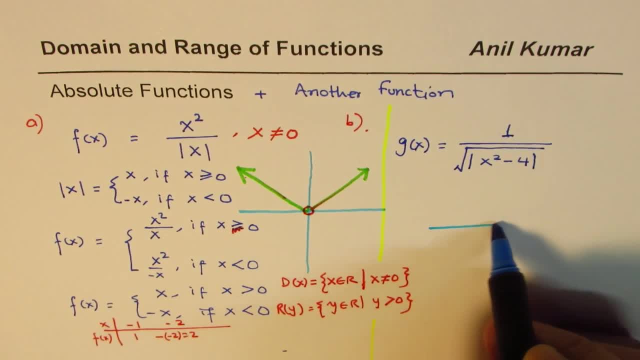 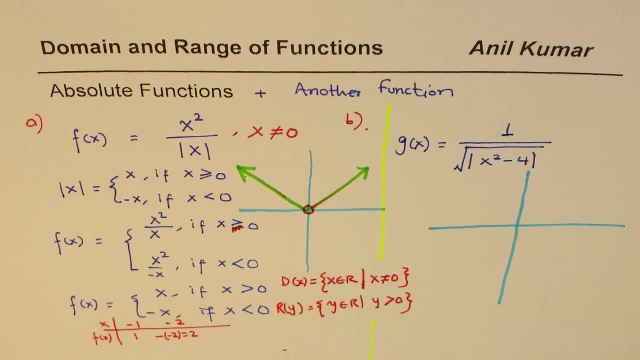 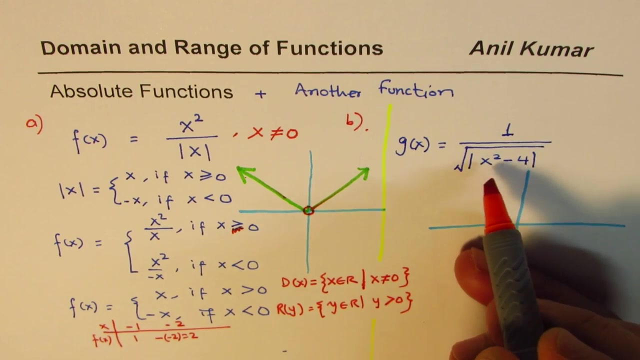 let me draw this line here. i think that bit of space should be okay. yeah, so this is our coordinate plane. so first i will start drawing with my inside function. okay, so the inside function here is x squared minus four. so x squared minus four is my inside function, which i am. 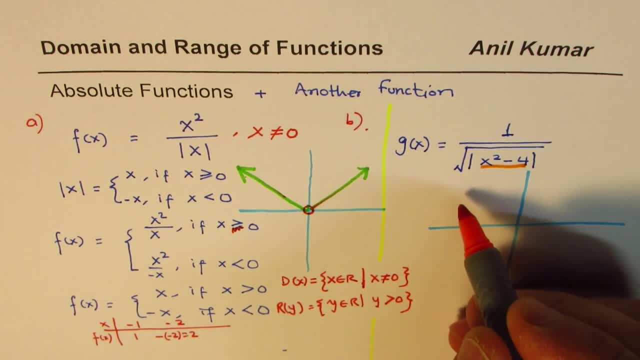 going to draw in this color. so this is a parabola, which will be kind of like this. so drawings are kind of approximate, but they give you a fairly good idea of what we're trying to do. so this function here is x squared minus four. okay, so let me write down here: this one is x squared minus. 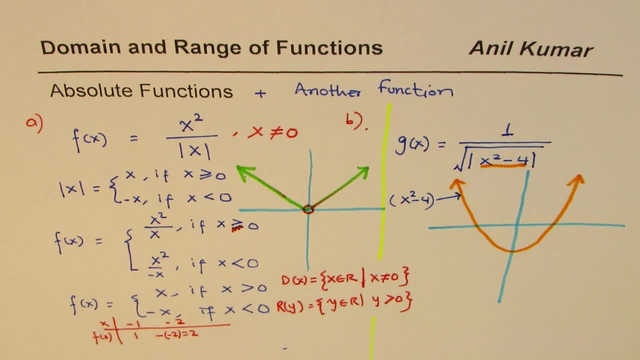 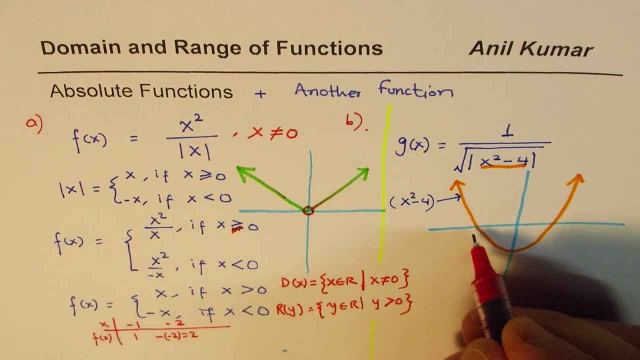 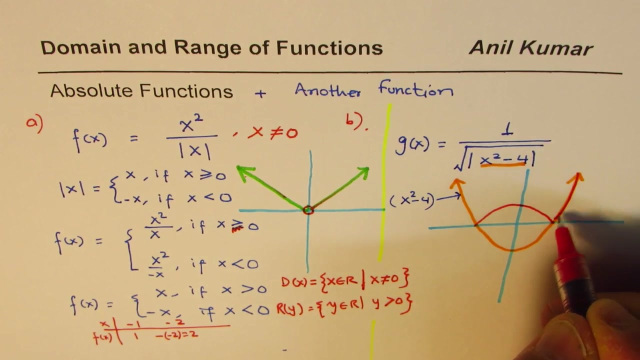 four. okay, this function. now, if i do absolute value of this function, then what it becomes? the negative part becomes positive, so it becomes like this: so this function which i am drawing now is the absolute value of x squared minus four. so this function is absolute value of. 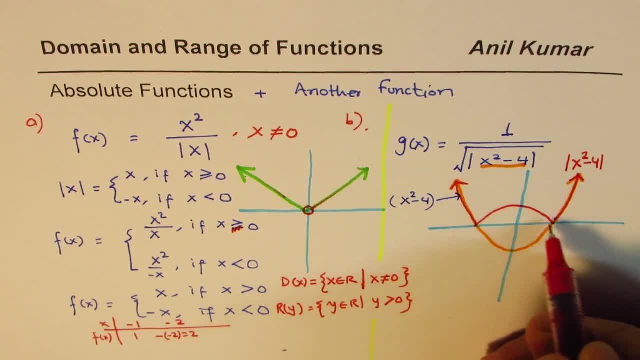 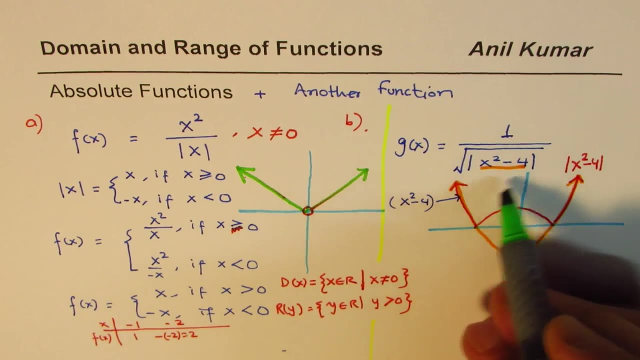 x squared minus four. it is always positive, as you can see, is it okay? okay, so this is the function here itself. now we'll draw this in green. this is the whole thing. so one divided by square root of this, correct? so? so let me draw one divided by this, or should i do square root part also? okay, so let me use another color, do square. 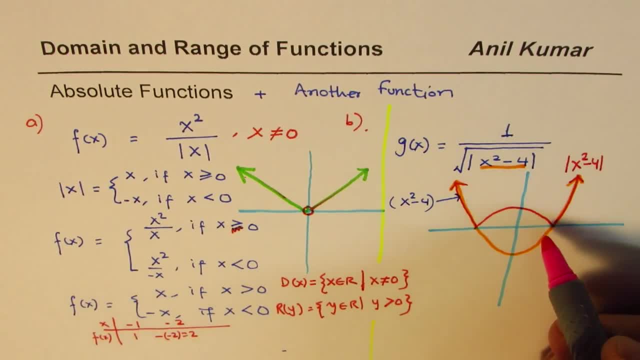 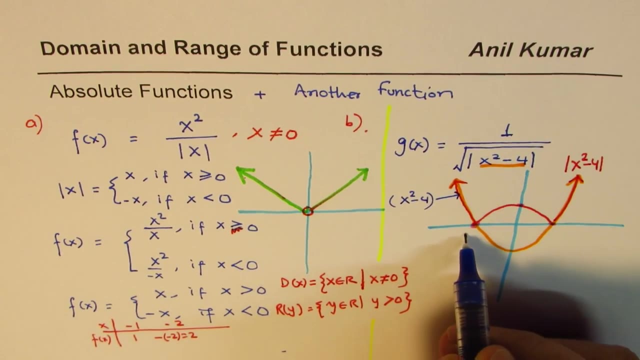 root part now. okay. so square root part here is that if i am at this point square root of zero zero, square root of zero zero, is that okay? now this point here is actually: let me number these: so x square minus one means this is minus two, this is two and this point here is a minus four. 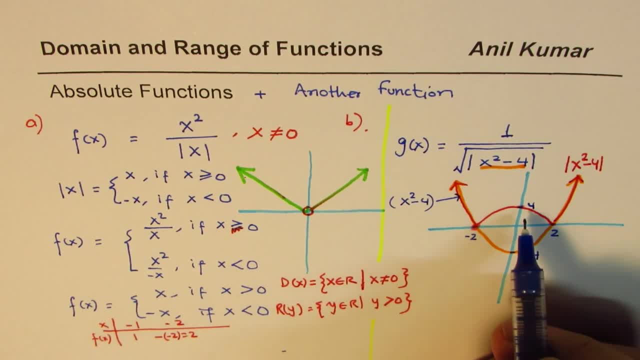 is that okay? so here, what we get here is four. square root of four is two. so we get a point here. it should have been further like this, but anyway, uh, let's say this is: this is two for us, okay, square root of zero is zero. square root of zero is zero. square root of four is two. 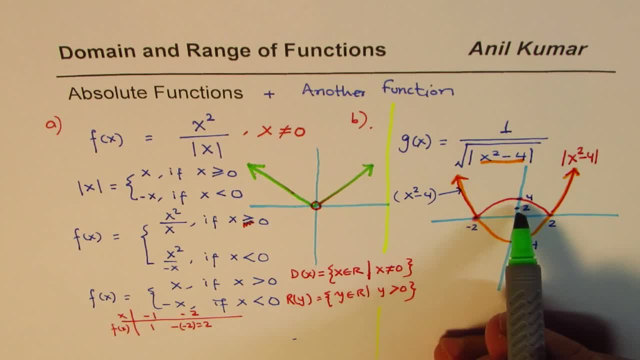 so in between we'll have values between zero and two. right square root of function is always increasing, correct? so here, if you go from here to there, the values are kind of decreasing. so from zero zero to this it is going to increase correct, kind of like this: here it is increasing in. 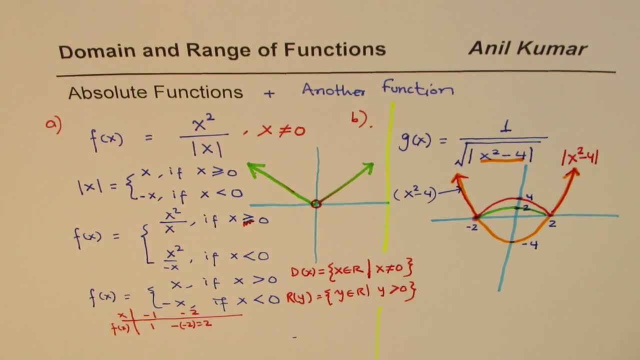 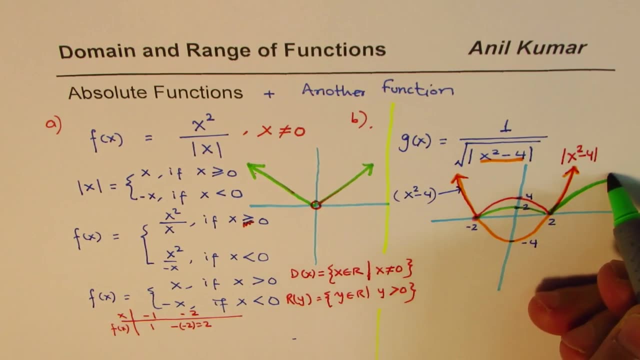 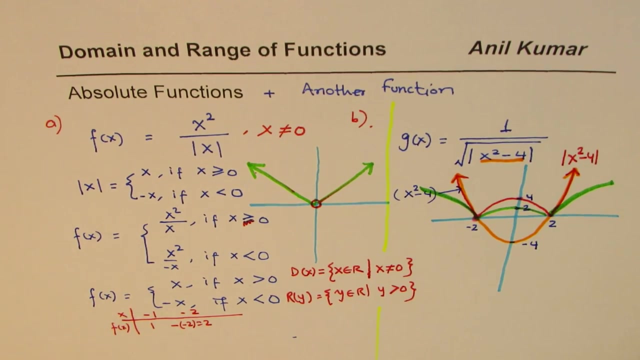 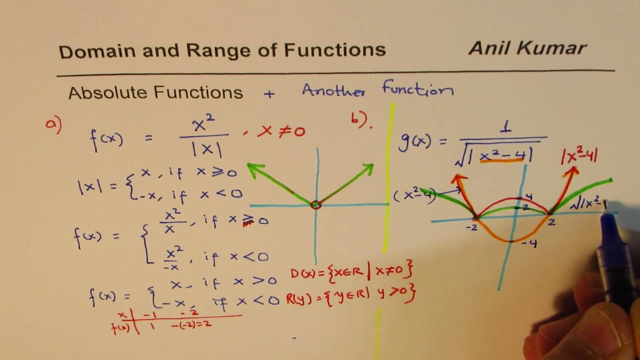 this direction. so so it looks like this, is it okay? so that becomes the square root function and since this value increases, square function will also increase, kind of like this. so that becomes the the graph for the square root part. okay, so what i have here is a function which is square root of absolute value of x square. 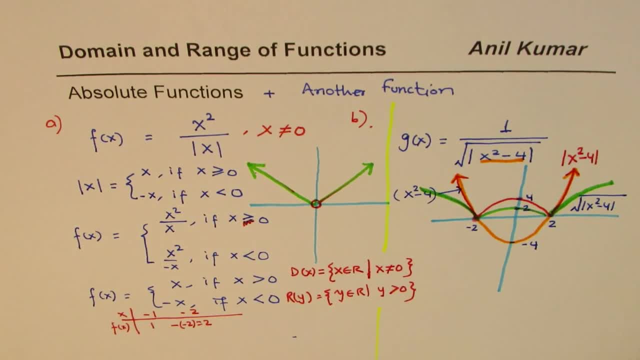 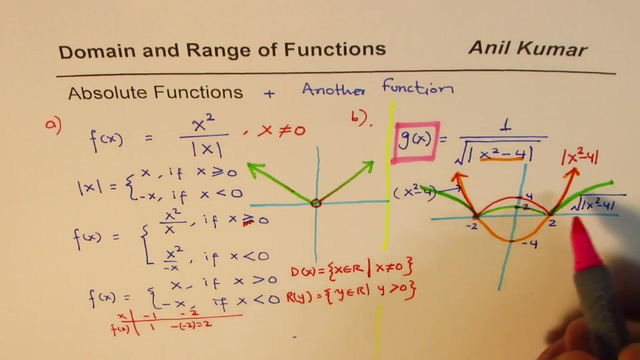 minus four. do you see that this is what we have and what are we interested in? one over reciprocal of this, reciprocal of this. so i need a different ink. okay, so we'll do with this one now. so now i'm sketching g of x, which is reciprocal of this green function. now. 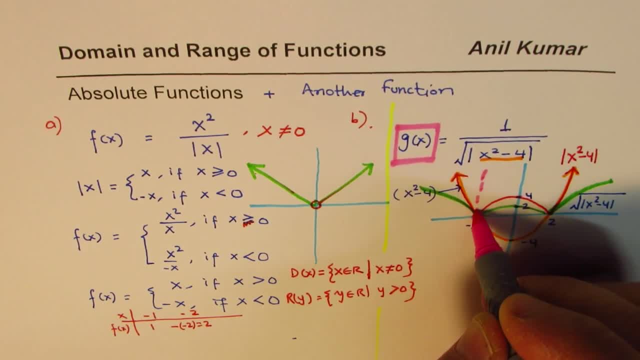 because 那 nosso什麼意思就是? at this stage, we'll have vertical asymptotes. do you see that we'll have helix? so we'll have vertical asymptote here, because they are zeros. anything divided by zero will lead to. 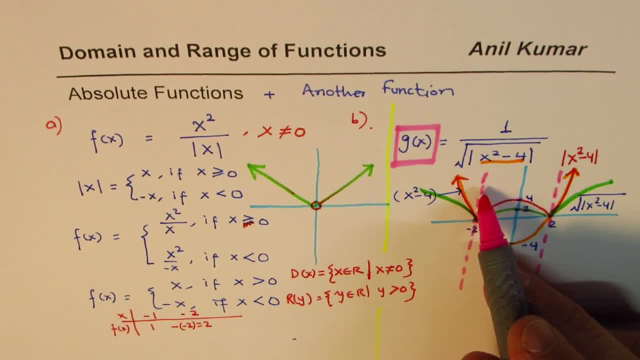 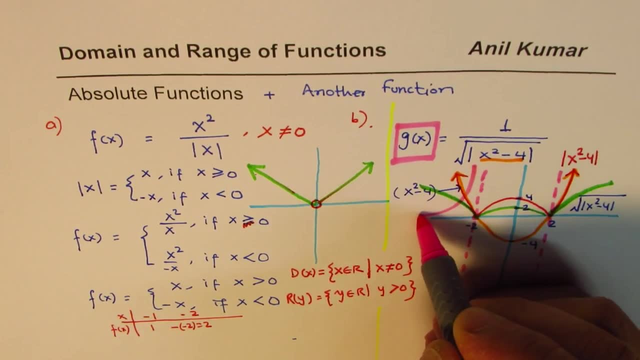 undefined value, which is resulting into a vertical s into now, since these values are increasing. here the graph will be kind of like this. let me just sketch the graph. we'll now not go into details for this, but i hope you understand and get it. so that is the graph of 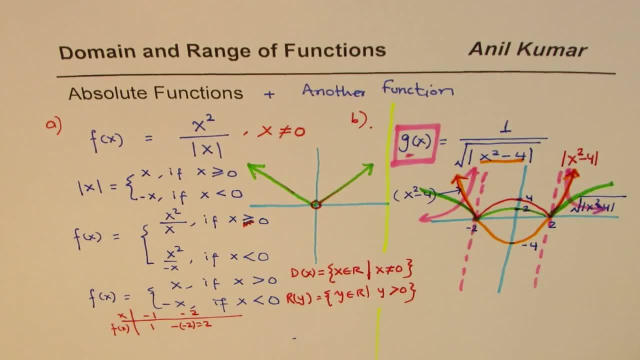 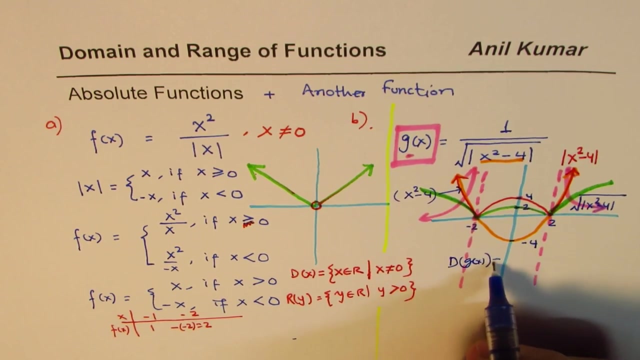 of the function g of x. So I hope that gives you a good idea of sometimes how complicated things could be in functions. right Now let me write down domain range for g of x. So we are considering domain of g of x, right? So, as you can clearly see, we cannot have 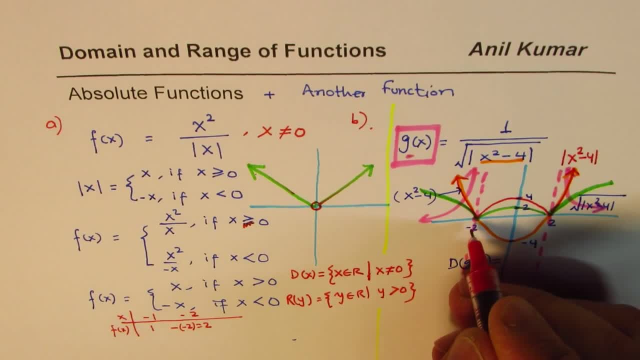 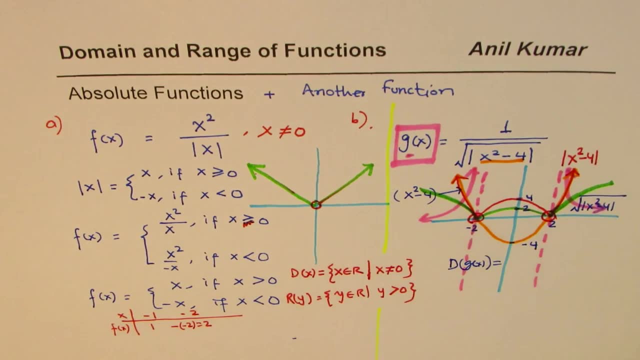 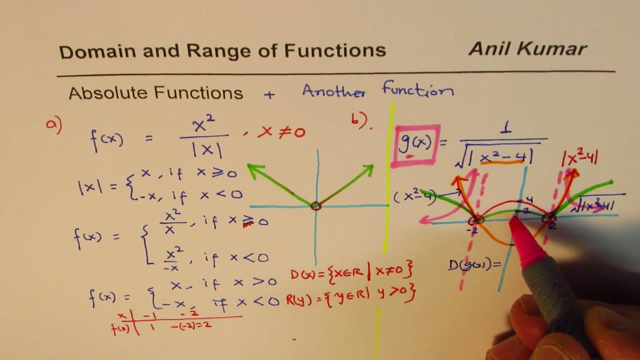 0,. I mean 1 over 0,, so this is not in the domain of the function. when you do square root, right, So this is out of the domain. and well, I did not sketch the center part, Let me do that also. So this center part here is this: value is 2, right, So square root. 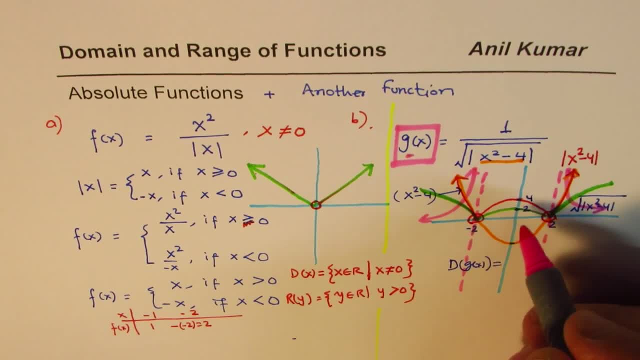 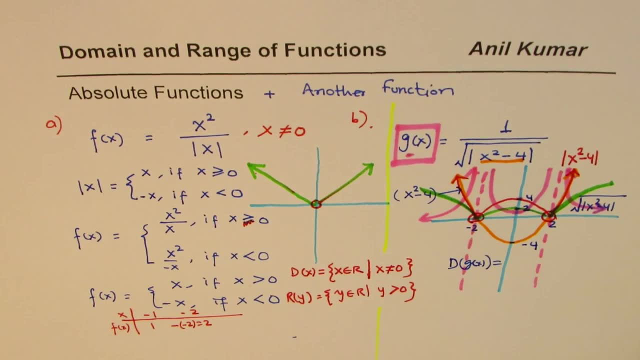 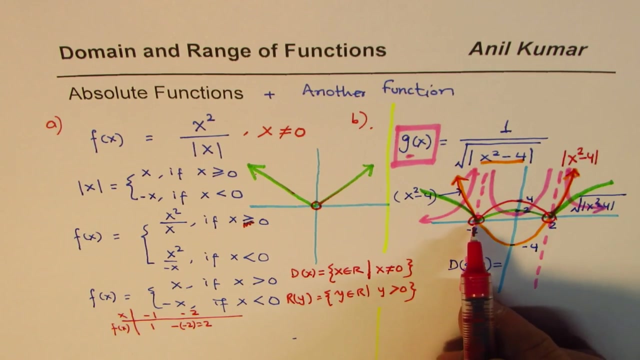 of 2 is something 1.14.. So this center part will be kind of like this. So let's say this is kind of like this: Is that okay? So what you really notice is that just g of x is always positive but greater than 0. But in the domain we will not include minus. 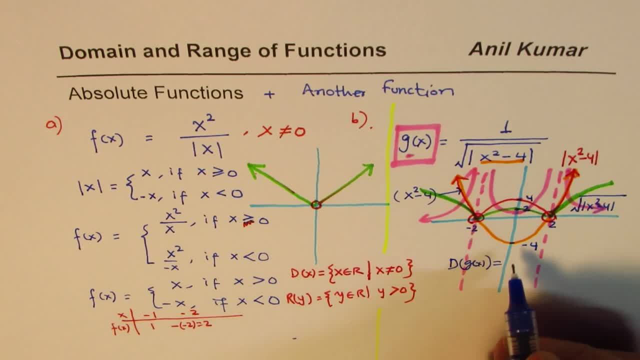 2. And plus 2.. So let me write down the domain of this function, which is x, belongs to real numbers where x is not equal to plus minus 2,. right Now that you could have got straight from the equation also, You don't really have to do all this. This is just to explain you. 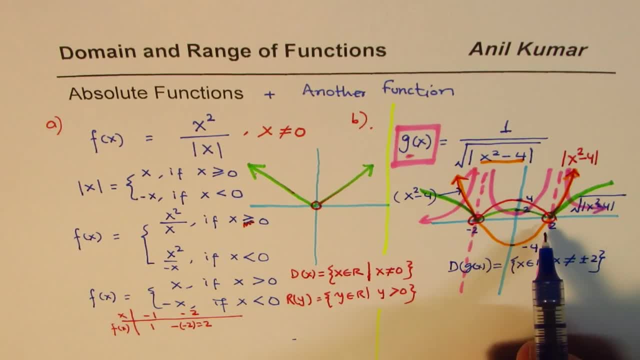 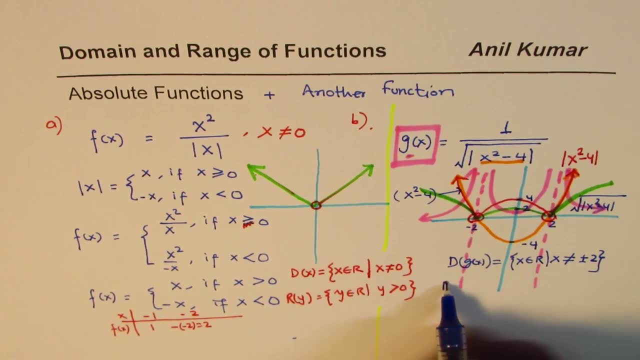 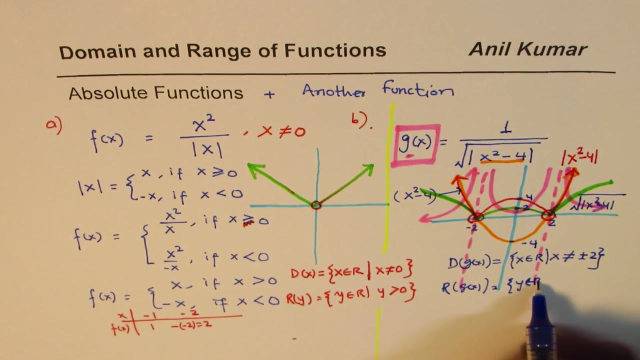 how to visualize it, which you may need in later half of this course. So denominator cannot be 0,. so straight away you get this domain. And as far as the range of this function, g of x is concerned, you can see it is y belongs to real numbers where 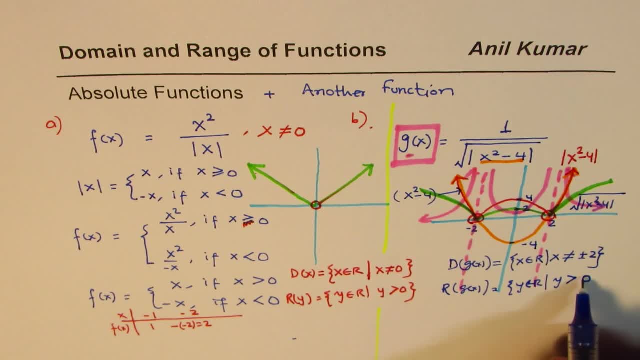 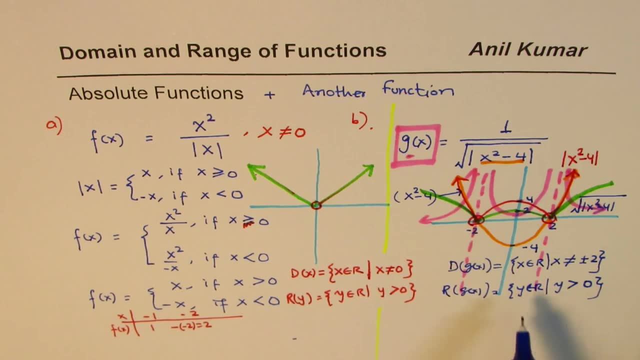 y is greater than right, It is always greater than 0.. So that is how you can get domain and range. Well, finding domain and range was not really difficult in this, since square root functions are always positive, Perfect, They are always positive right, And so reciprocal.